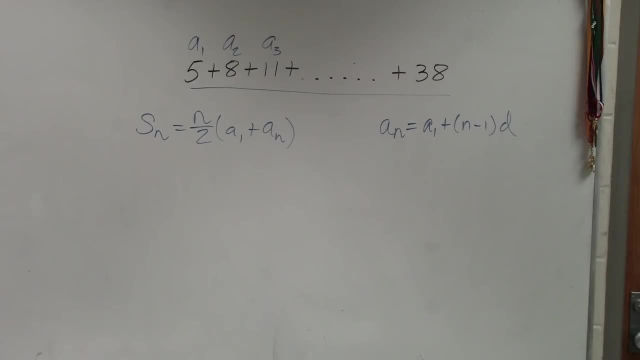 You are going to be constantly using that formula. Any time you have an arithmetic sequence you're going to want to remember, pull out this formula and think about it. So let's look at this. What information do we have? The thing that we have is: we know a sub 1, which is 5.. 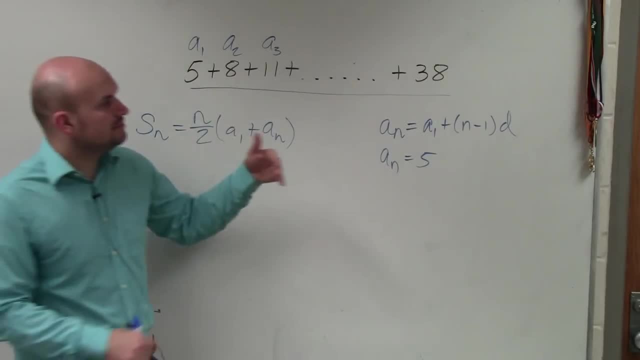 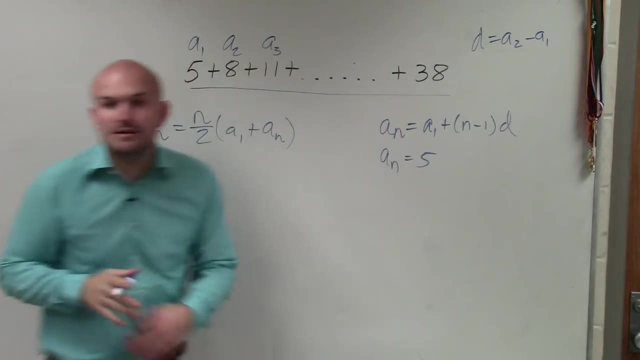 And do we know what the difference is? Crystal, this is not helping your case right now. Wow, you're always complaining. a sub 2 minus a sub 1, okay, If you guys look at this, remember the difference: a sub 2 minus a sub 1, it has to be the same for all the terms. 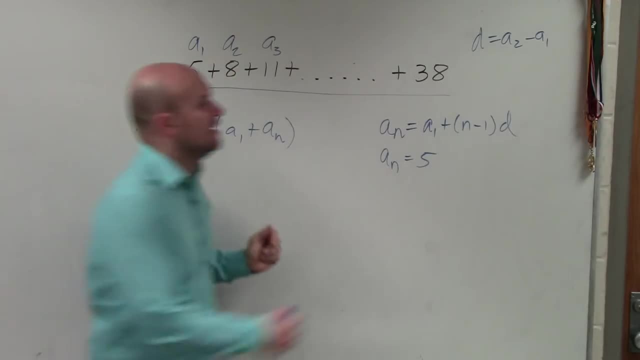 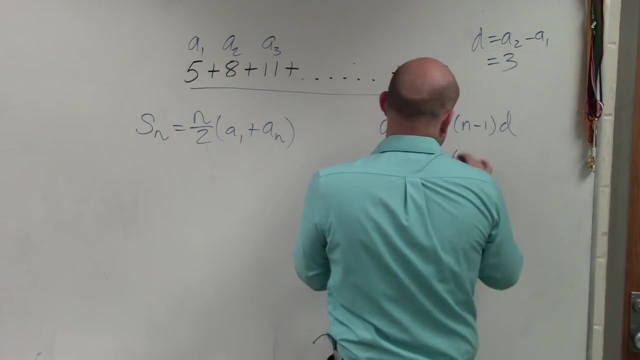 So if I do a sub 2 minus a sub 1,, I do 8 minus 5, which is 3.. And then I want to make sure: is 3 the common difference between all the terms so far? Yes, So I can say a sub 1 times n minus 1 times 3.. 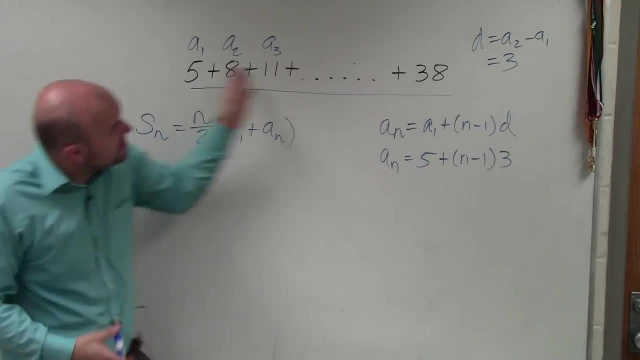 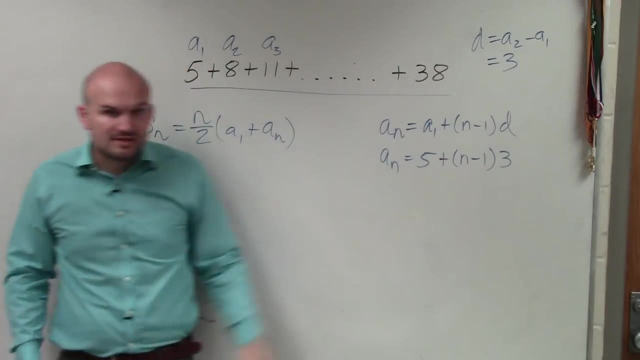 Now I don't know n, right, N tells you, Sinan, the number of terms in this sequence. We don't know n, but we know a sub 1, which is the first term, and we know the difference. 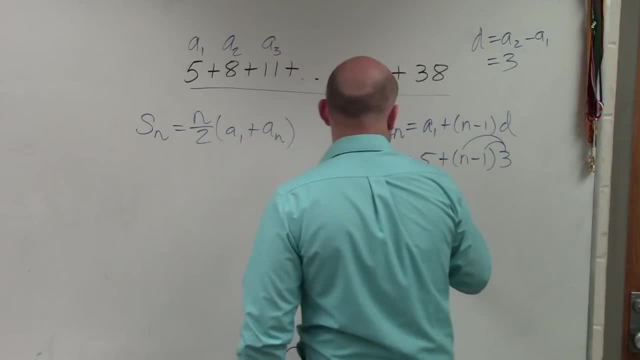 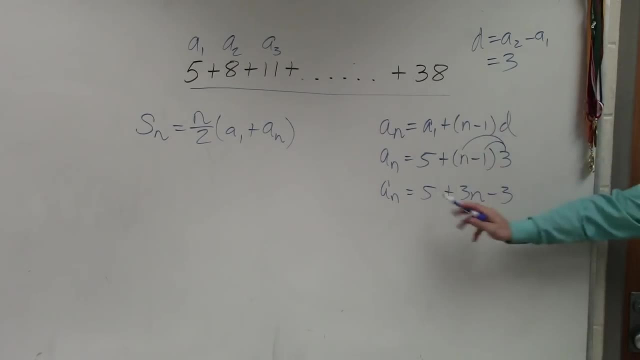 So now what I'm going to do is apply distributive property: a sub n equals 5 plus 3n minus 3.. Now I combine like terms: 5 minus 3 is 2.. So I can say a sub n equals 3n plus 2.. 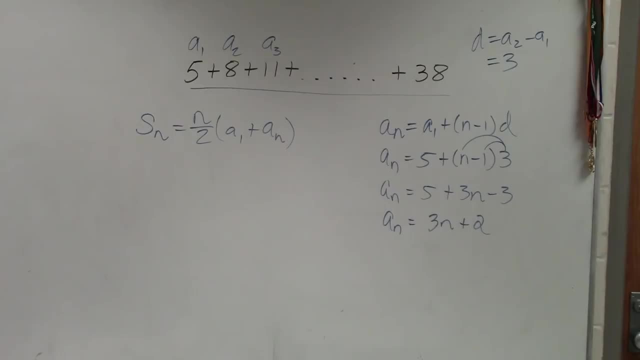 Anybody have any questions on how I got to that point so far? No, Okay, So now again, what is it? we don't now remember guys, remember when I gave you, remember the first day we talked about sequences. 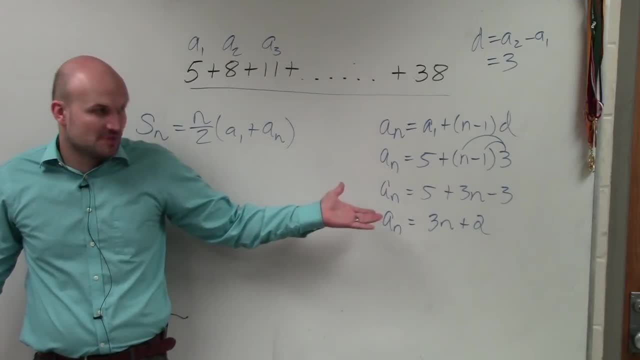 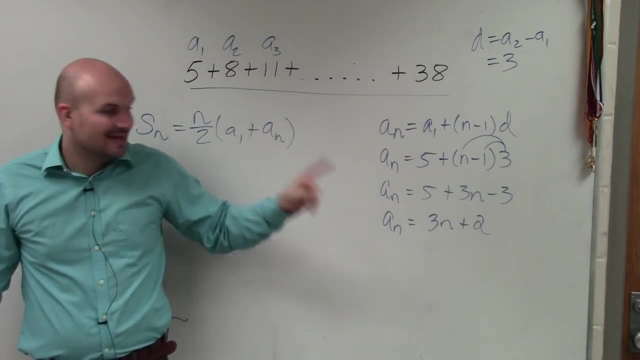 I said, hey, find the first five terms right. Remember we did that. What do we do to find the first term? We plugged 1 in for n right, in this case n. And if I said: what's the second term? 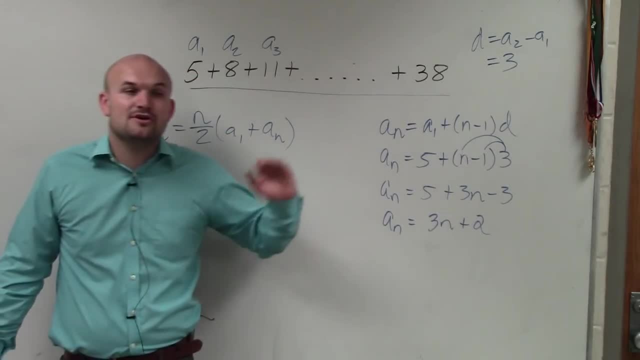 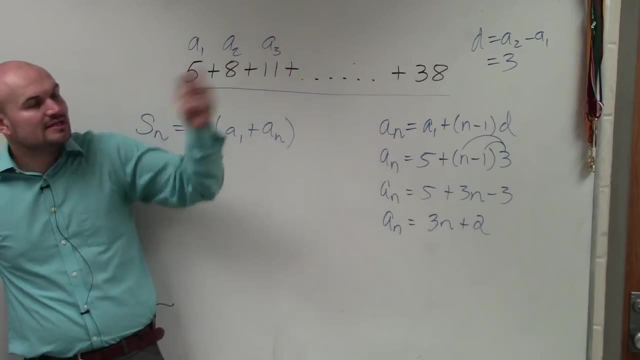 You plug 2 in for n, And then I say 3, the third term, you plug in n. You kept on plugging in n. right, Oh, you kept on plugging in what? What number in the sequence? Yes, Chris huh. 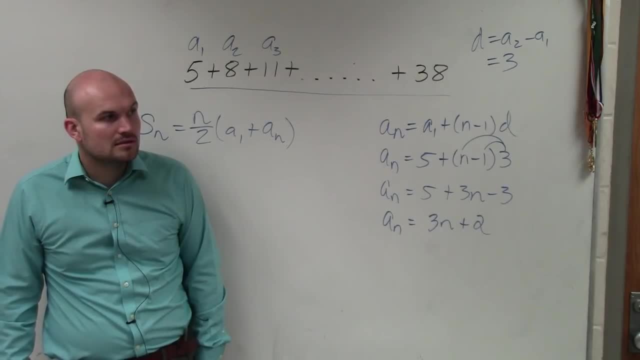 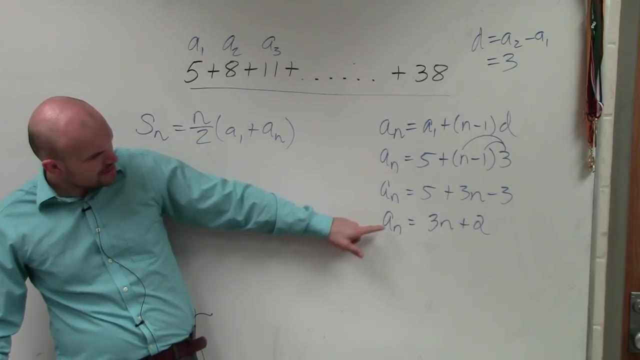 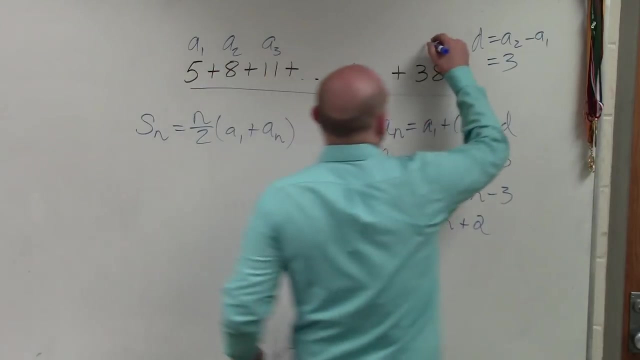 Okay, fine, I'm going to go over the answers on the test. that's cool In this case, so so the thing that we do not know, though, is: we don't know what number term this is. We don't know, we don't. this is a sub n, for all we know, right. 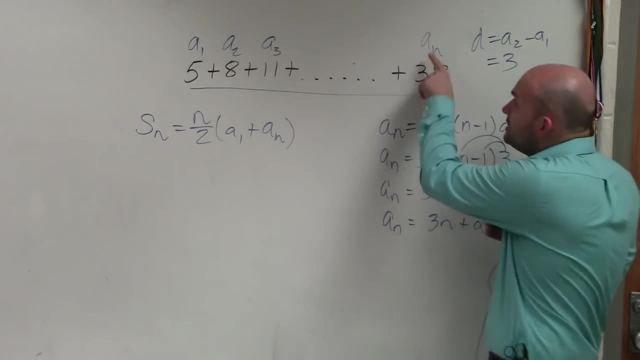 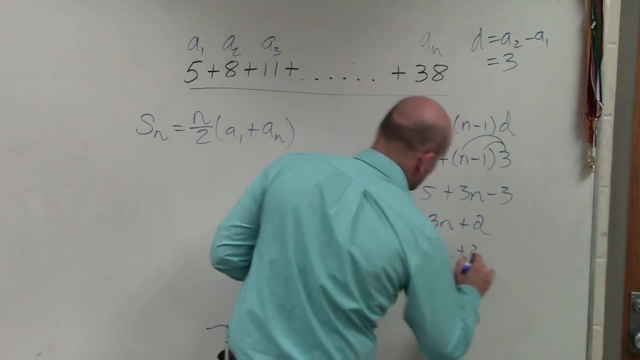 We don't know what number this is going to be, So what we're going to have to do, we know that a sub n is 38. We just don't know what n is, So I'm going to plug in: 38 equals 3n plus 2.. 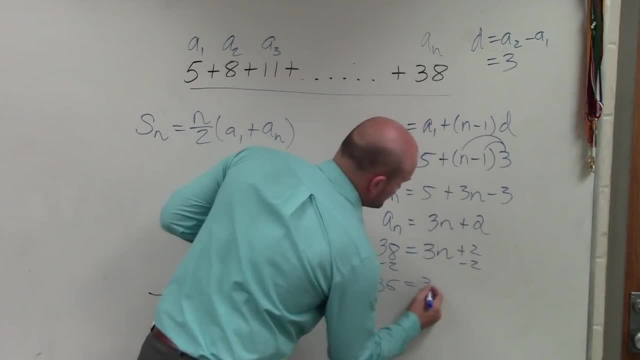 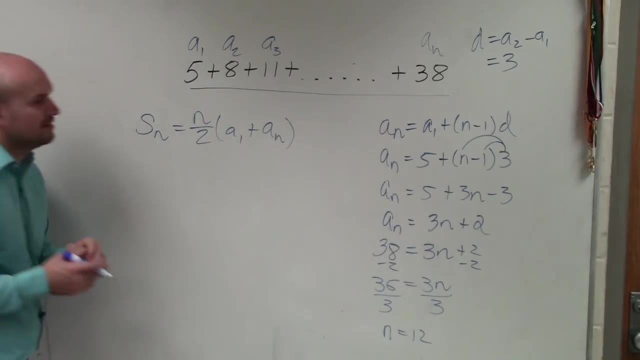 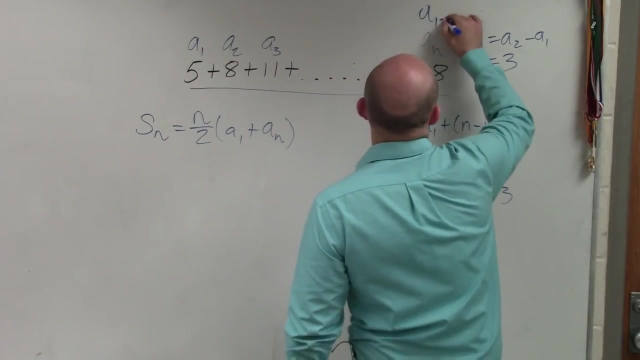 I'm going to subtract the 2 and get 36 equals 3n. divide by 3,, divide by 3, and I get n equals 12.. Now that's very, very important, because now I know that this is not a sub n. this is now. 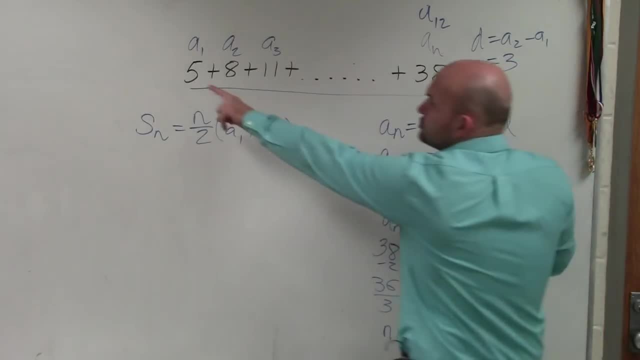 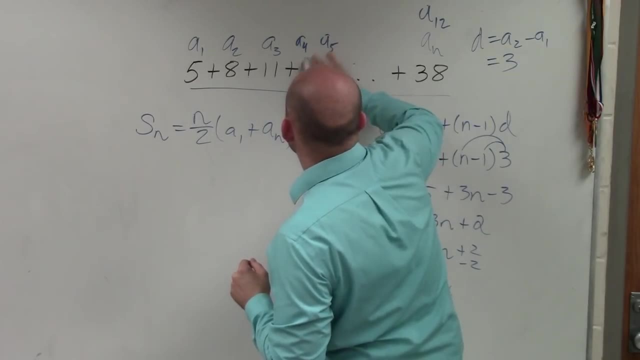 a sub 12, right, Because I know now there's 12 terms. If you were to keep on counting, that's by 3, right 14.. If you were to keep on counting, a sub 12 would be 38.. 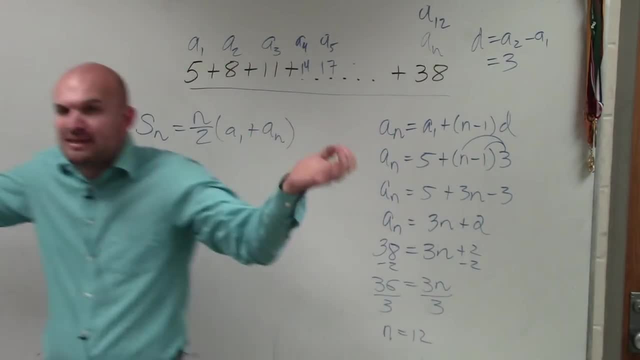 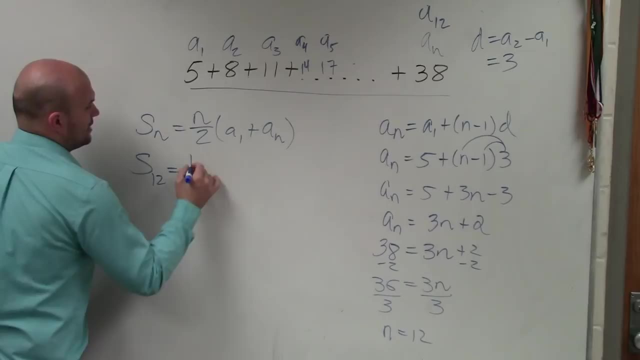 Because now to do the sum, you have to know what n is, You have to know how many terms you're finding the sum for. So the sum of 12 terms is going to equal 12 over 2 times a sub n. Okay, 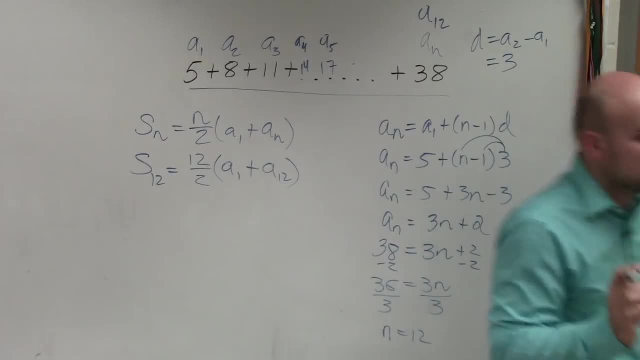 A sub 1 plus a sub 12.. All I did for the first step was just plug in 12 in for n. Do you guys see how I, whatever I plugged in for whatever I replaced, since I replaced 12 in for n, I replaced that everywhere. 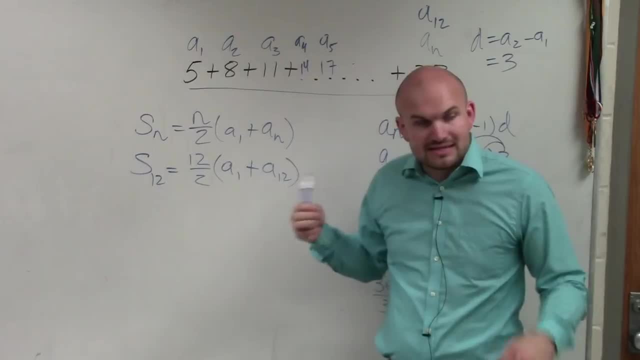 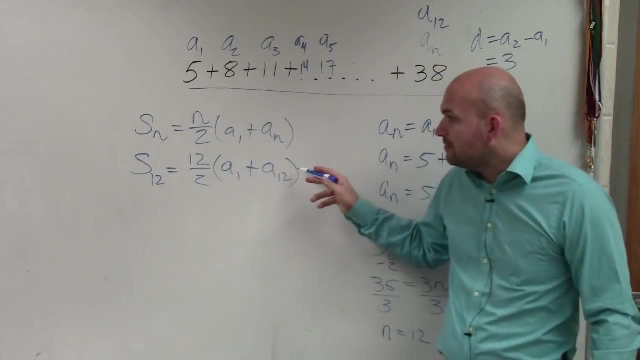 You guys see that, Because n represents 12, now N represents the number of terms. We know the number of terms is 12.. So now do I know what a sub 1 is? 5. Do I know what a sub 12 is? 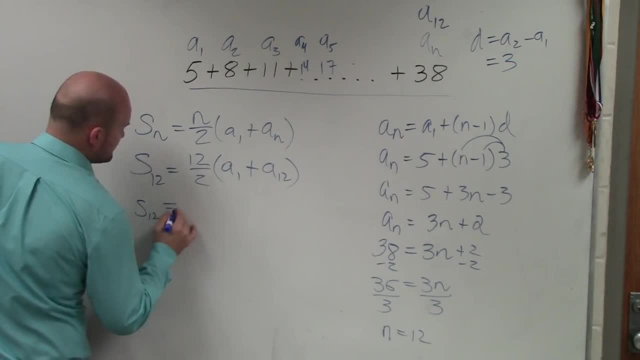 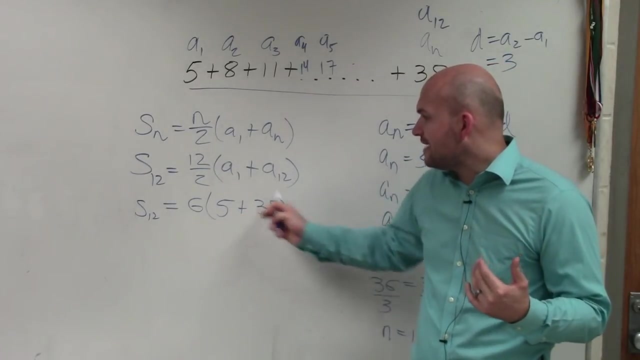 Yeah, So now I do a sub 12, or s. sub 12 equals: 12 divided by 2 is 6, times 5 plus 38.. Now all I simply need to do is add. I use my distributive property. 5 plus 38 is going. 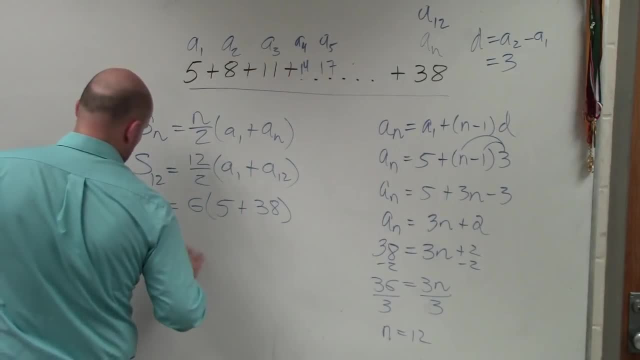 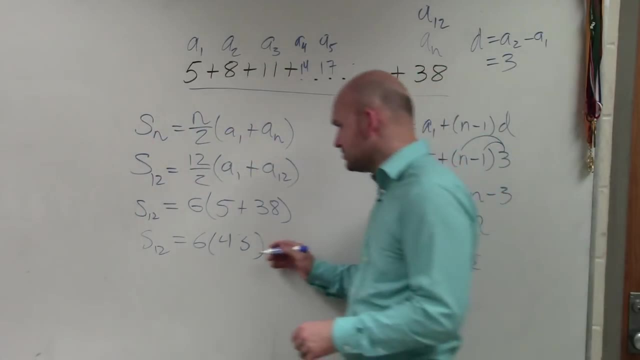 to be a 43. And then I go ahead and multiply, which would be 258.. If you guys want to check my way, My work, please. That's too much. How do we know if you're not lying to us? 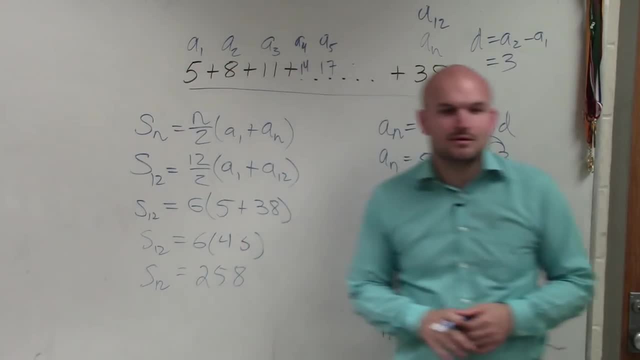 That's why he said we can check his work. Yeah, please check my work, Giselle. how many times have you gotten like mad?